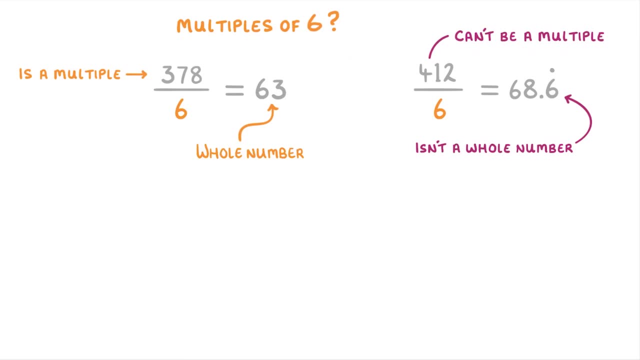 of 6.. Another way to think about the multiples of a number is to just keep on adding that same number. So to find the multiples of 14, we could just keep adding 14.. So you get 28,, 42,, 56,, 70, and so on, And all of these numbers that we 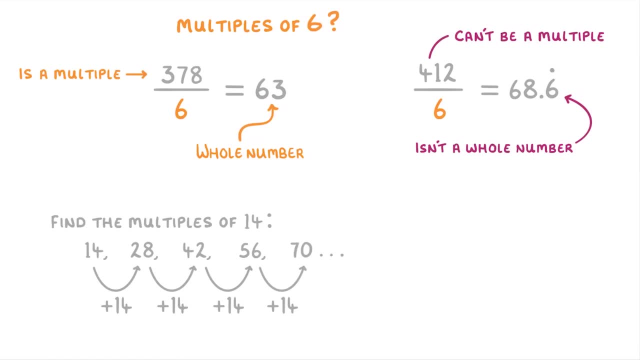 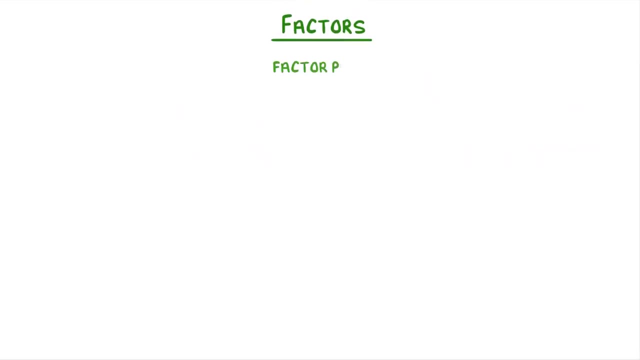 get would be the multiples of 14.. Now the best way to understand factors is to start with factor pairs. Let's take a look at all 8 numbers first. If we had the number 28,, then its factor pairs would be the pairs of whole numbers that can be multiplied together to make 28.. So 2 times 14,, 4 times 7,. 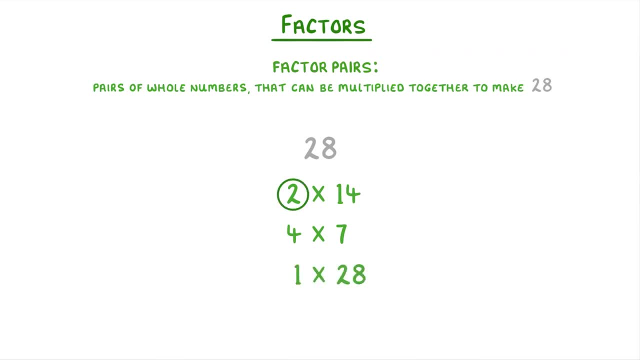 1 times 28.. And if these 6 numbers that make up these factor pairs, that would be the factors of 28.. because they're all whole numbers that can be multiplied to Berlioz's. Colonel simple defines it by another whole number to make 28.. 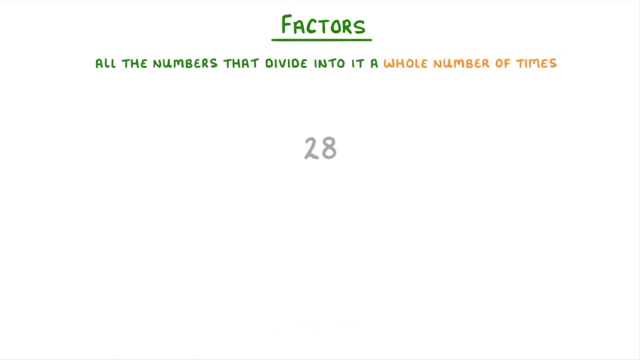 Another way to think about the factors of a number are all the numbers that divide into it a whole number of times. For example, 4 is a factor of 28, because 28 divided by 4 is 7, which is a whole number, Whereas 5 isn't a factor because 28 divided by 5 is. 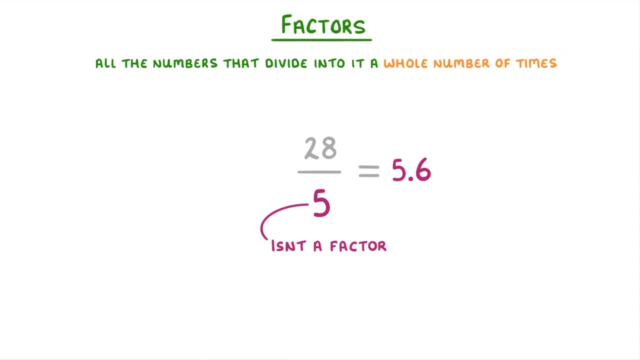 5.6, so 5 doesn't go into it a whole number of times. If you want to quickly find all the factors of a number, the best thing to do is write out all the factor pairs Starting with 1 times the number at the top. 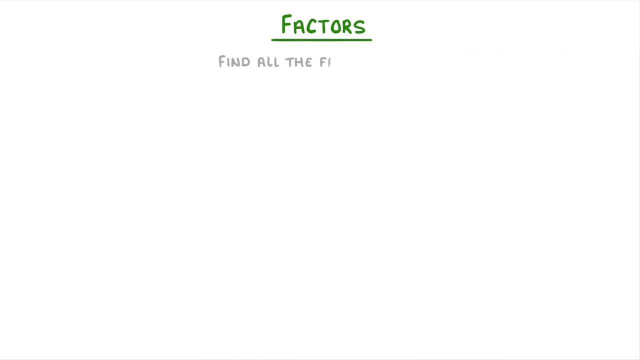 So if we want to define all the factors of 48,, we'd start with 1 times 48,, then do 2 times whatever factor is needed to make 48,, so 24, and so on with 3 times 16,, 4 times. 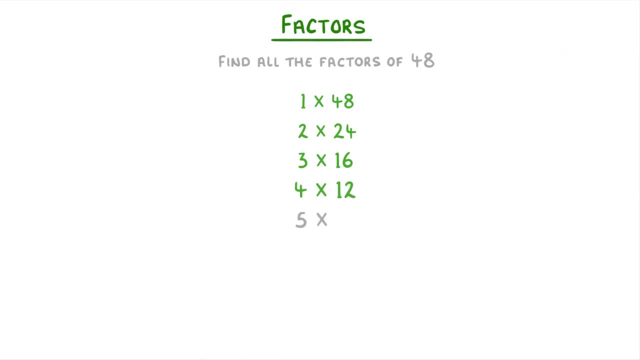 12,. 5 doesn't go into 48,, so isn't a factor. then we have 6 times 8,, 7 times 8, and so on. 1 also isn't a factor, and so on, and so we get to 8, which we've already covered in 6 times 8.. 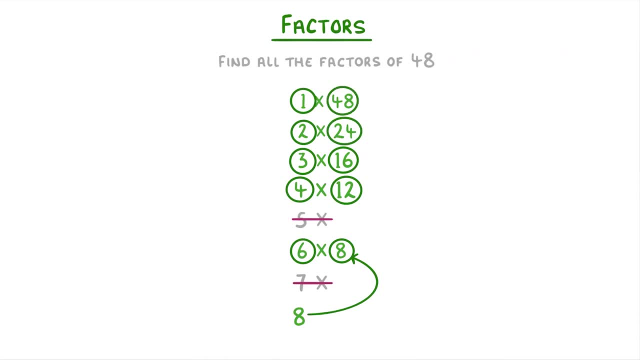 We stop here. Our ascending order is 16, d1, b1,, b2, d3, d4, d5, and d8.. 1-2-3-4-6-8-12-16-24-48-願-Has- subconsciously gone- Libertarian. And so we know that our factors are 48, d1, and d4, d4-d4,, d5, and 74, and so on. If you want to make a multiply guess, come to maintenantcom ormia d1,- d4,. obj orisis D1,. 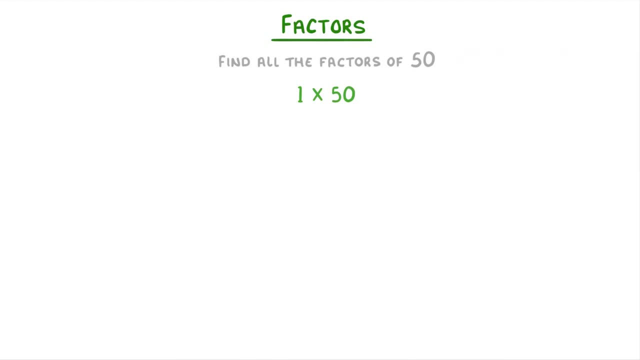 Etter entr Stones go into an project of a number you're a member of. we're to do 1 times 50,, 2 times 25,, 3 doesn't go into 50,, 4 also doesn't work, 5 times 10, 6,, 7,, 8, and 9 don't work. and then we're at 10, which we've already done. 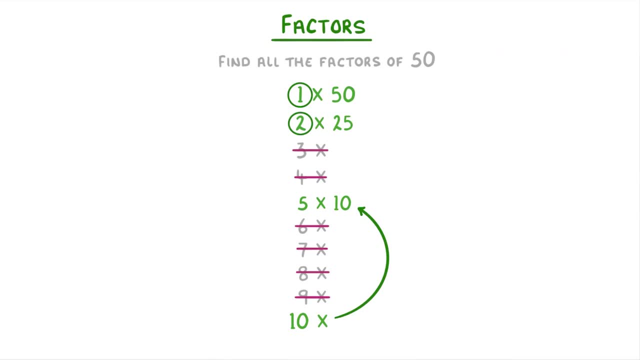 So the factors are just 1,, 2,, 5,, 10,, 25, and 50. So, to quickly sum everything up, if we took a number like 12, its multiples would be the bigger numbers that it can multiply to, like 24,, 36,, 48, and so on, whereas its factors 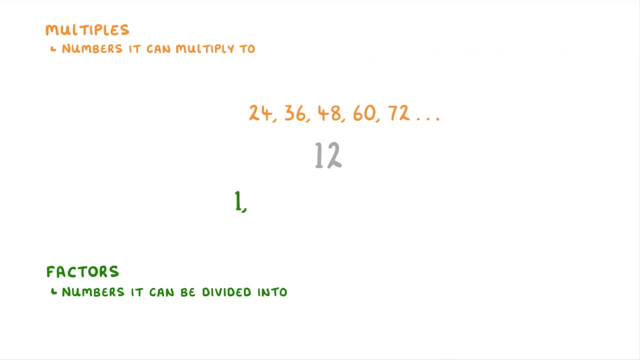 are the numbers. it can be divided into like 1,, 2,, 3,, 4,, 6, and 12.. Just make sure that you remember which one is which, Because it's really easy to get them the wrong way around in the exam. 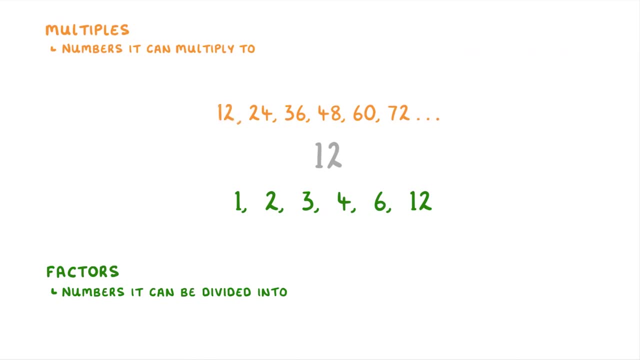 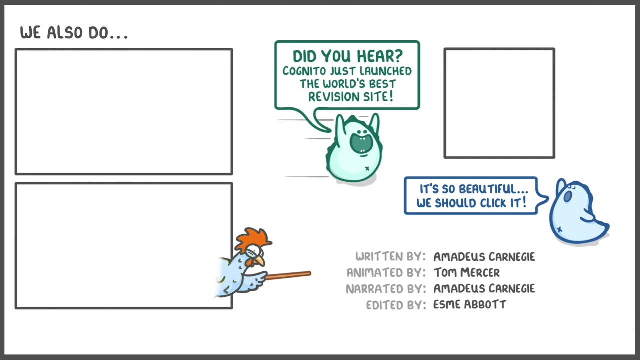 And also remember that the number itself counts as both a multiple and a factor, So 12 is in both of these lists. Anyway, that's everything for this video, so hope you enjoyed it and we'll see you next time. Subtitles by the Amaraorg community.